So here it would just be 12 times 4,, which is 48 units squared. So for that one we're going to be 12 times 25, which is 300 units squared for out new area of k, And then this will be 12 x 25 present units for 1.. This will be unlike the previous 서eda limit. 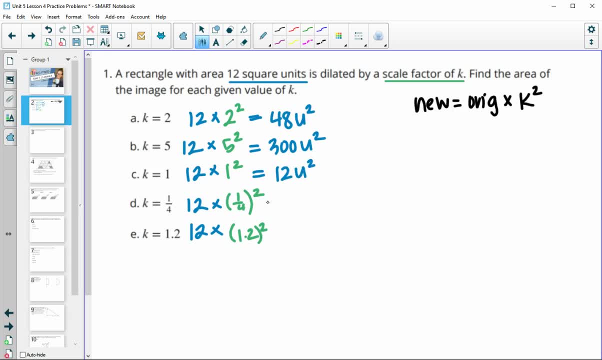 be 12 times 1, so just 12 units squared. since it didn't change in size at all, This one will be 12 times 1, fourth squared, which is really like dividing by 4 twice, And so this one as a decimal will give us 0.75 units squared. And then this final one, 12 times 1.2 squared. 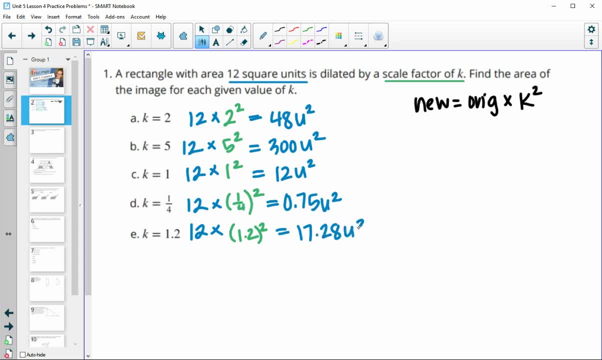 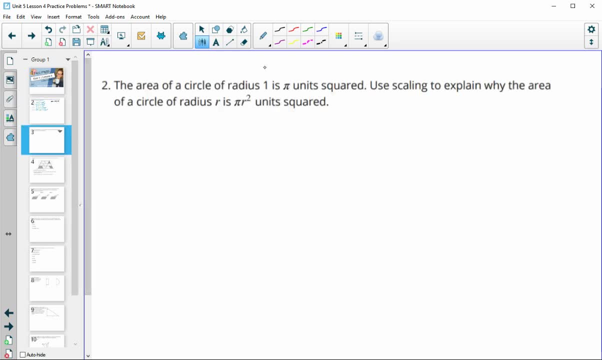 is 17.28 units squared. Number two: the area of a circle with the radius of 1 is pi units squared. Use scaling to explain why the area of a circle with radius r would be r units squared. So remember what we just did in the last one is our. 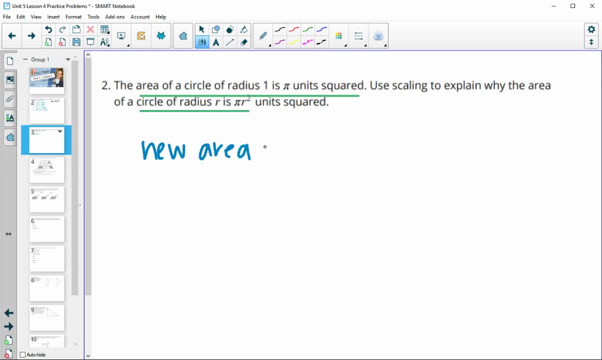 square root of 1.2 squared. So we're going to use scaling to explain why the area of a circle would be r units squared. So remember what we just did in the last one is: our new area is equal to our original area times the scale factor squared. So in this case, 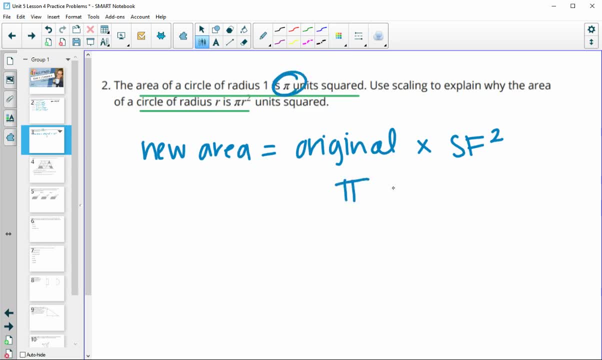 our original area is pi And then our scale factor. since we went from a radius of 1 to a radius of r, our scale factor is going to be the new dimension divided by the original. So our scale factor is going to be the new dimension divided by the original. So our scale factor. 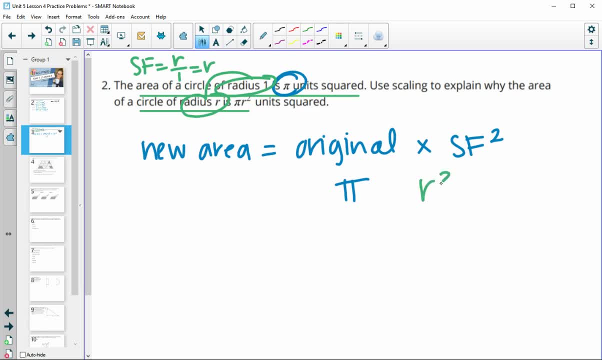 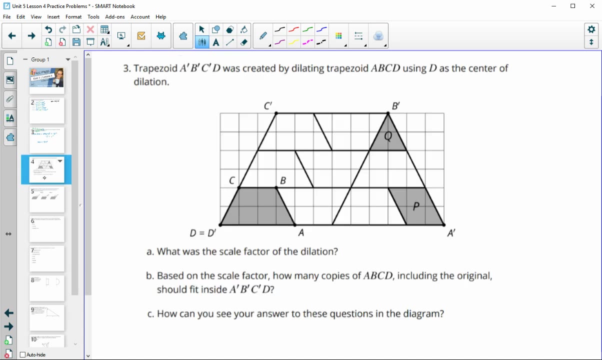 is going to be the new dimension divided by the original. So our scale factor is r, So we're going to be multiplying by r squared, And so then we can see that our new area is going to equal pi times r squared. Number three: trapezoid: A, prime, B prime, C prime, D prime. So this big trapezoid was created. 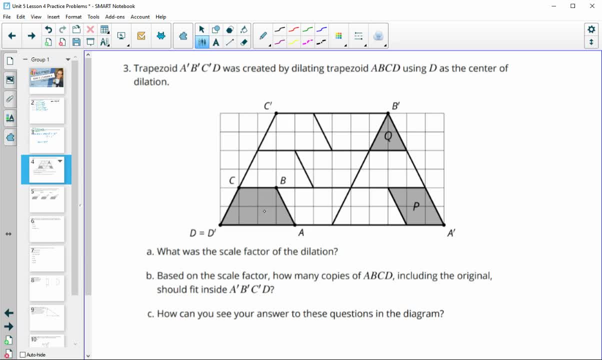 by dilating ABC, this little one down here, Using D as the center of dilation. What is the scale factor? And so we can see that we're going to this larger shape. Let me get this to be a little bit thicker. So here's A prime, B prime. 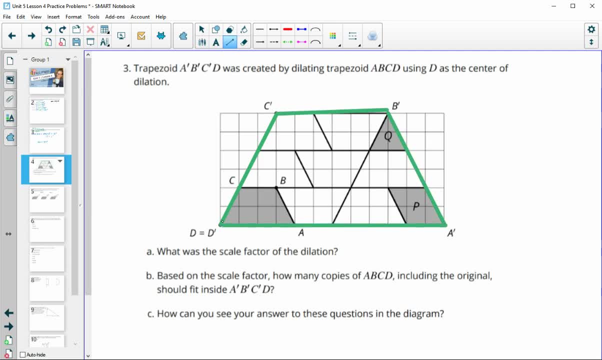 C, prime, D, prime. So here's our larger trapezoid And then so we just kind of want to see how many times does this smaller one fit into that. So if we take a look at this smaller one here, so how many times could we fit? 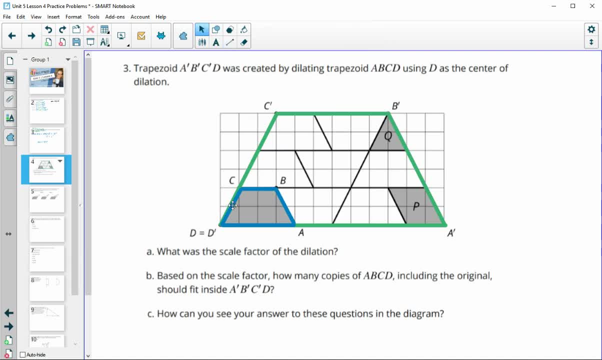 this in each dimension, So you want to see how the dimensions change. So I'm just going to be looking at this side So we see that this goes once, twice, three times. So this green length, okay, is three times bigger than the original. So the scale factor is: 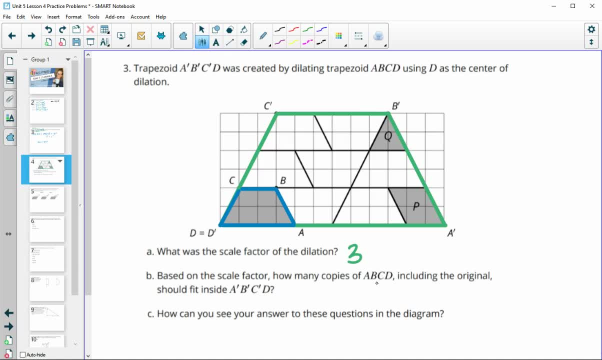 three, Based on the scale factor, how many copies of ABCD, including the original, should fit inside? So this is talking area. So this is going to be the scale factor squared amount of times, So nine times, And you can see one, two, three, four, five, six, seven, eight And then 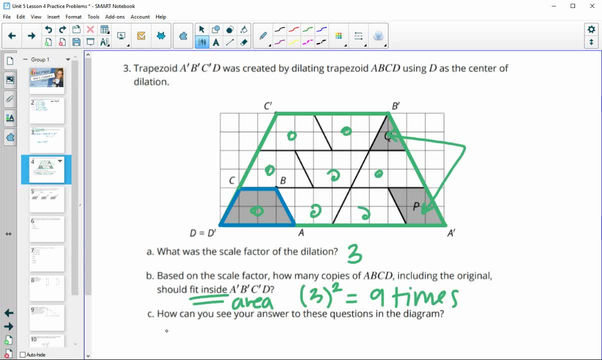 this piece connects together to make the ninth. How can you see these answers, the answers to these questions? So we just kind of talked about the first one and then the second one, So you can see that the last one is the same as the one in your diagram. So we just kind of talked about that last one And 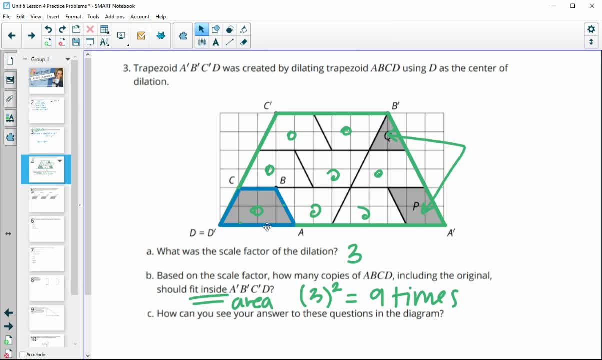 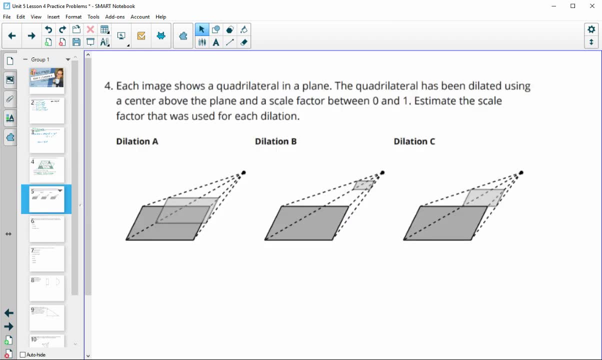 then also the original, that this just fits three times up the side length or three times across the bottom. If you wanted to take this and move it, you could get it three times in there again. Number four: each image shows a quadrilateral and a plane. The quadrilateral has been dilated using the center above the plane. And then a second image shows the center above the plane. So that's our quadrilateral image for this. All right, so let's take a look at this. So we just kind of talked about that last one And then also the original. 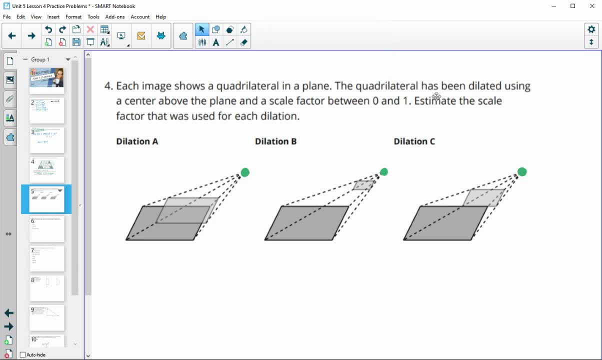 and then a scale factor between zero and one. So estimate the scale factor that would be used. So this one looks like about halfway, This one is kind of a scale factor less than a half, so probably a fourth, And this one is between a half and one. 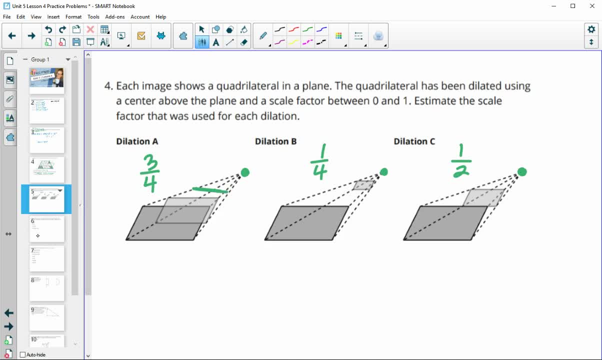 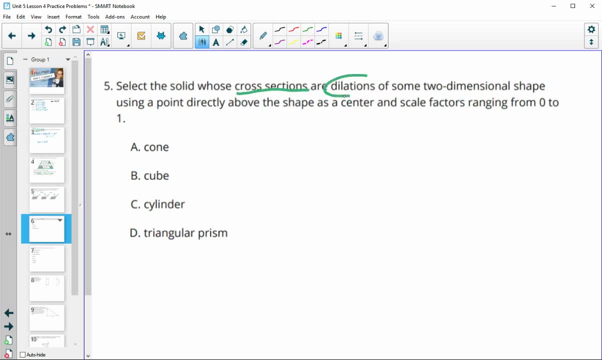 so something like three-fourths for that one, All right. number five: select a solid whose cross sections are dilations of some two-dimensional shape, using a point directly above the shape as the center and scale factors from zero to one. So this is meaning that it's going to be getting smaller. 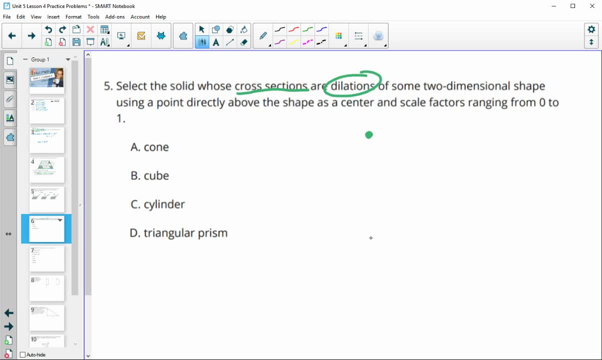 as we go up to this point. So we have some shape down here, dilations all the way up to this point, disappearing to this point. So that would work for a cone. So if you have a cone, so a cone would just be circles, okay. 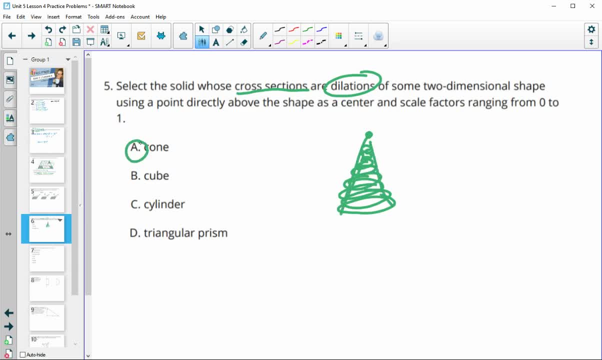 down up until we got to that point. So a cone would certainly work here. A cube would not, because a cube is just going to be the same cross sections over and over and over, all the way up to the top, and they're going to stay the same in order to make that cube. 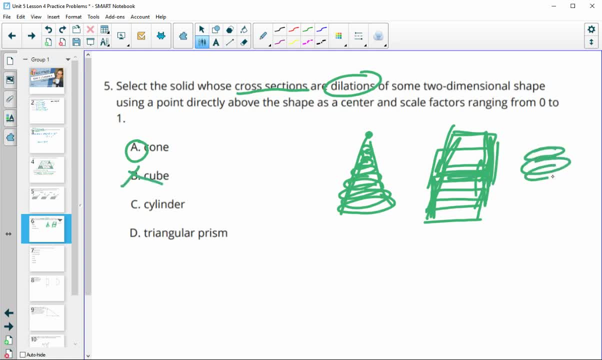 So cube would not work Cylinder either, because a cylinder is just going to be the same cross sections all the way from top to bottom, Since it stays uniform the whole way, And same with the triangular prism. okay. So prism means it's going to be a triangle at the top. 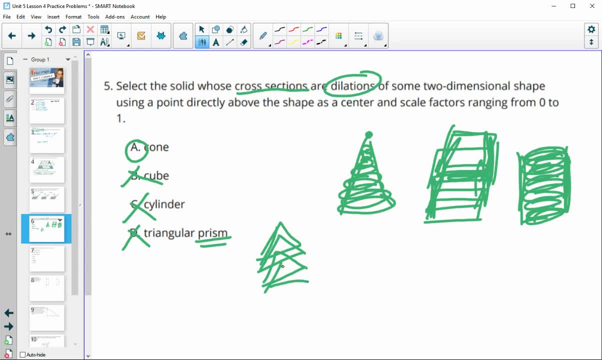 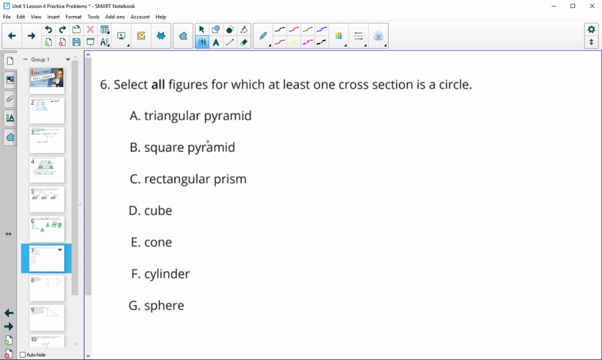 and the bottom. So this is just going to keep doing this all the way from top to bottom to stay uniform in size. Number six: select all figures for which at least one cross section is a circle, So a triangular pyramid would not, because that's going to have. 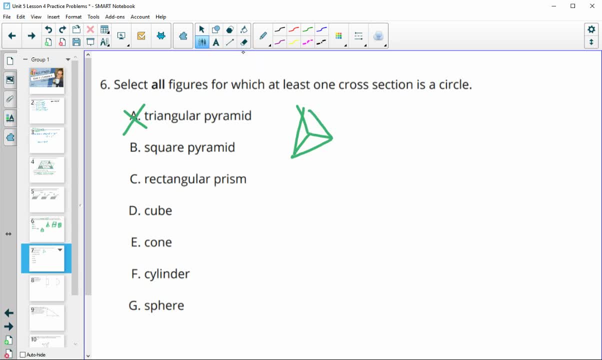 a triangle at the bottom and go up to a point. So all of the other ones are going to be triangles as well. So square would be either squares or triangles. Rectangular prism is going to have rectangles from bottom to top, So it's going to be- you're going to have rectangles. 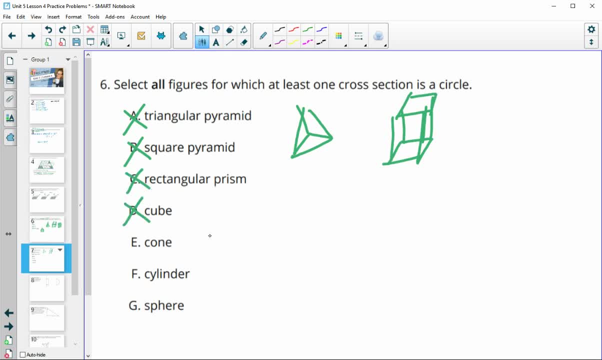 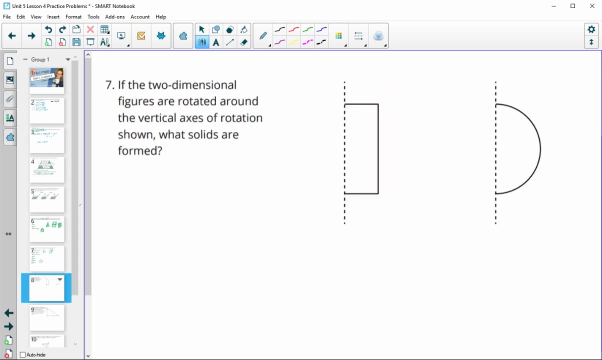 or squares, for that one Cube would be all squares. A cone has a circular base, So that one would be good. Cylinder has a circular base, and then sphere has circular cross sections around it. for sure, If the two-dimensional figures are rotated around the vertical axis. 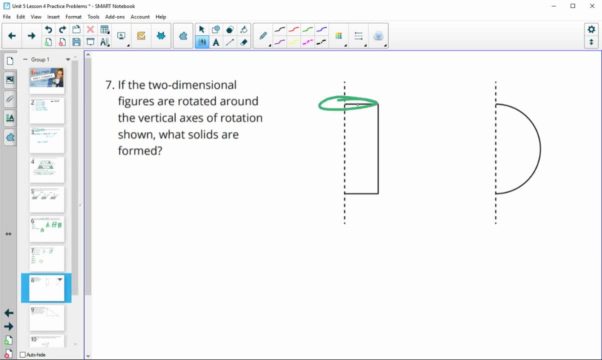 shown what solids are formed. So remember that it's going to go circular, right. So it's going to rotate around here, So we'd end up with this. So this one's going to be a cylinder, Okay, and this one's going to rotate around here. 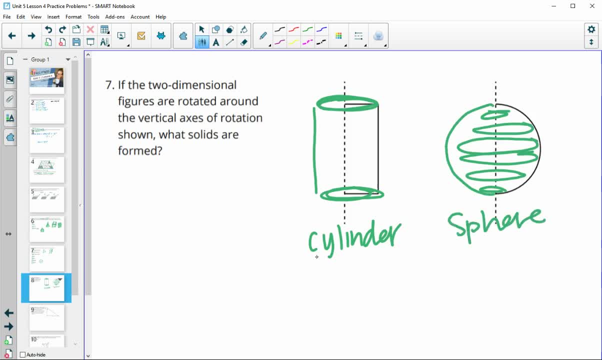 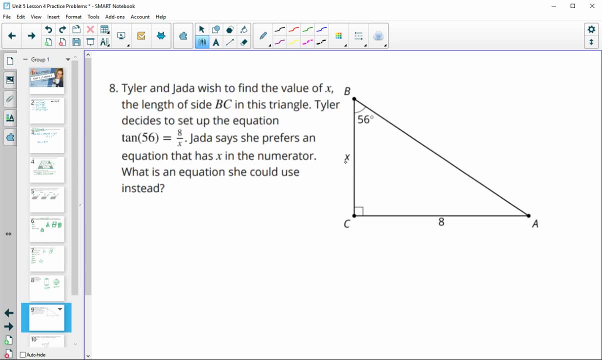 So this one, you're going to get a sphere. It's going to be the same thing. So the two-dimensional figure is going to be a cylinder. So this one's going to be here. Number eight: Tyler and Jada wish to find the value of X in the triangle. 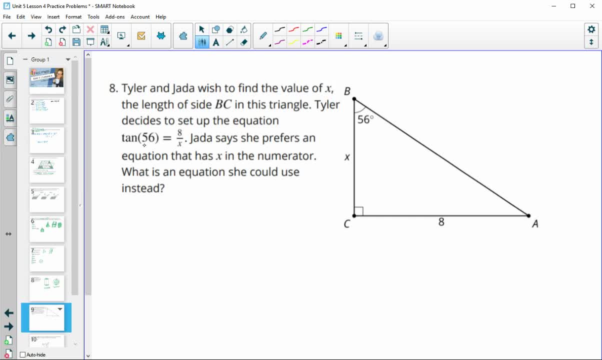 Tyler decides to set up the equation. the tangent of 56 equals eight over X. Jada says she would prefers an equation with the X in the numerator or in the top. What equation could she use? Okay, So Tyler used the 56 given. opposite is eight divided by adjacent. 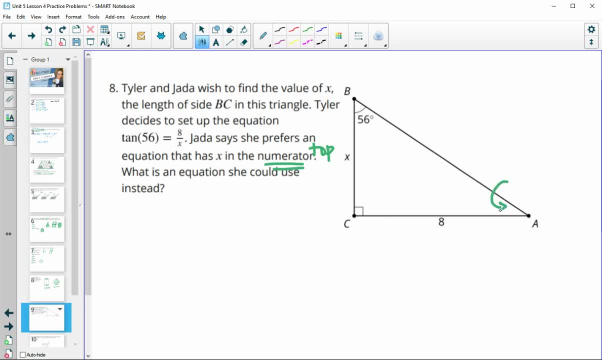 So Jada is going to use the 56 given. opposite is eight divided by adjacent. were to use this angle here, okay, which is going to be 90 minus 56 or 34, Jada could do a tangent function. So tangent of 34 is equal to the opposite, which is X over the adjacent eight. 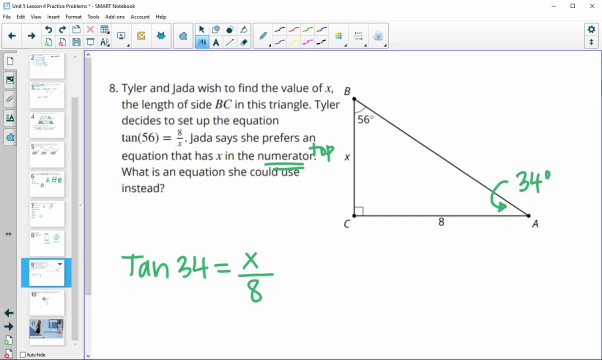 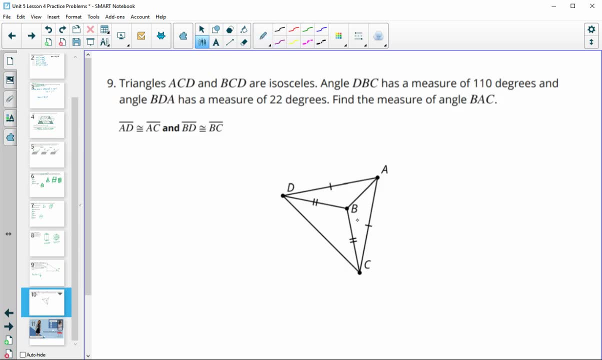 So she could use that equation instead. All right. number nine says the triangle ACD and BCD are isosceles and we see those marked on this picture. Then it says angle DBC, So this angle here is 110 degrees, And angle BDA, So BDA, this angle here has a measure of 22 degrees. 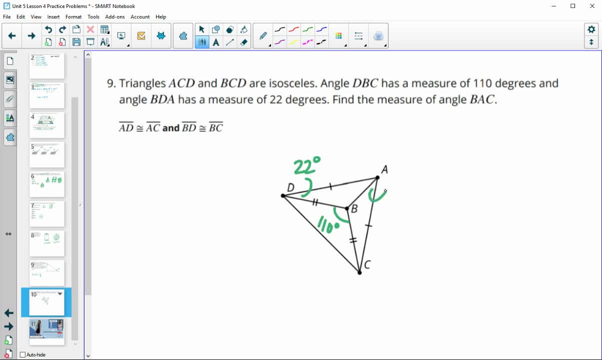 Find the measure of angle BAC. So ultimately, we want to know this angle here. All right, So let's take a look at a couple of things here. So remember that we have an isosceles triangle here, So this angle here is going to equal this one. So if we were to take 180 and subtract 110 from it, 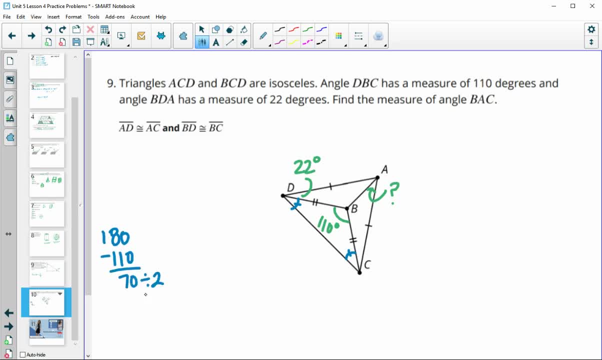 we would get 70. Then we could divide that by two to get 35 degrees for each of these angles. We also see this segment. AB is in both of these two triangles over here. That would mean that these two triangles are congruent by side side side. Okay, so we know that each of these